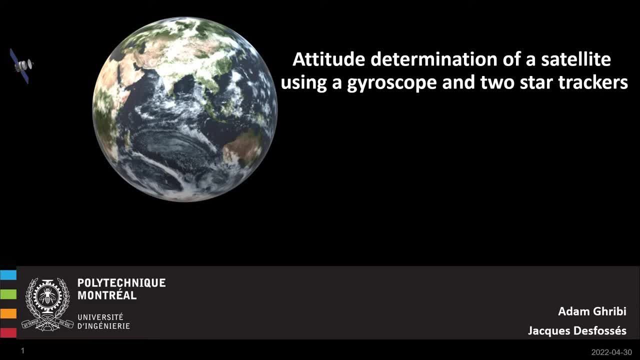 Hello everyone and thank you for watching. My name is Jacques Defausse and my colleague's name is Adam Griby. Today we're going to discuss about our navigation system project titled Attitude Determination of a Satellite Using a Gyroscope and Two Star Trackers. 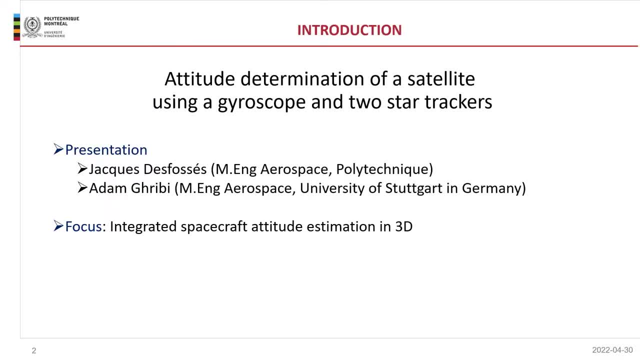 Adam and myself are both master's students in aerospace engineering. Adam is an exchange student from Germany and I'm from Polytechnic. We're both passionate about space, and that's the reason why we've decided to focus on a project where we determine the attitude of a spacecraft. 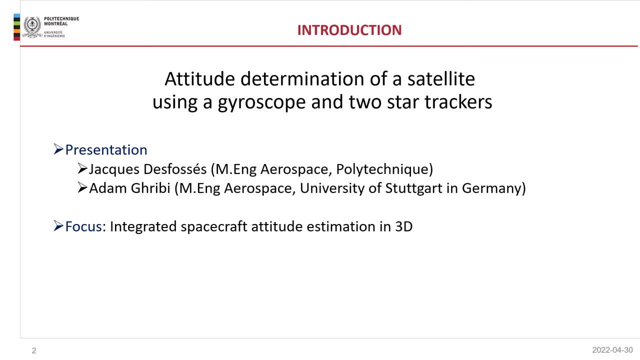 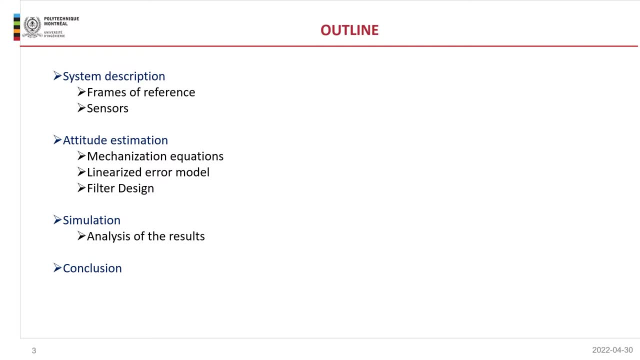 in 3D. Navigation systems are critical in space and we wanted to know more about them. This presentation is split as follows: We're first going to describe the system, the frames of reference and the sensors, and then we're going to move to the heart of the problem: the attitude. 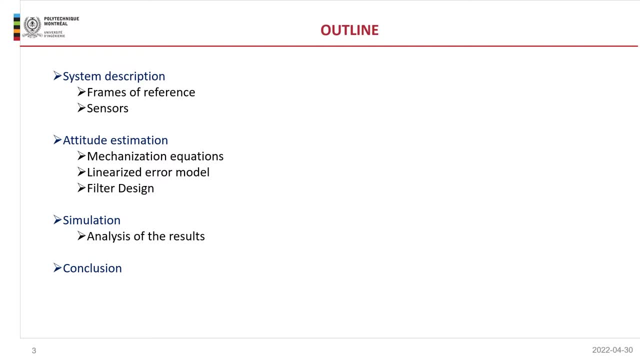 estimation, the mechanization equations to linearize the room model and the filter design. Afterwards, we're going to discuss how we're going to design the system, the frames of reference and the sensors. Afterwards, we're going to discuss how we're going to design the system, the frames of reference and the sensors. 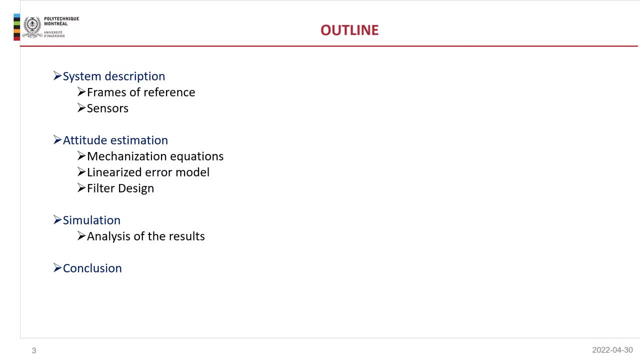 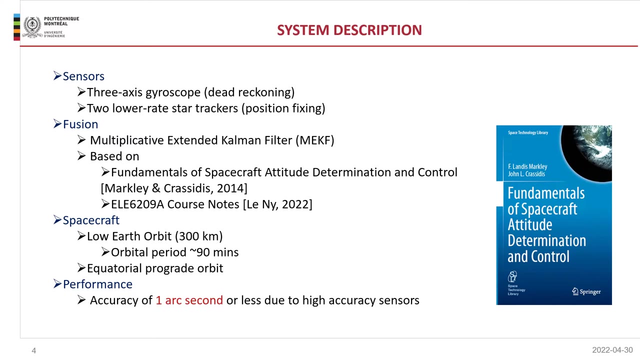 We're going to talk about the simulations that we performed on the system and we're going to discuss about the results that we obtained, and we're going to have a short conclusion afterwards. Our system has two types of sensors: one 3-axis gyroscope for dead reckoning and two lower rate. 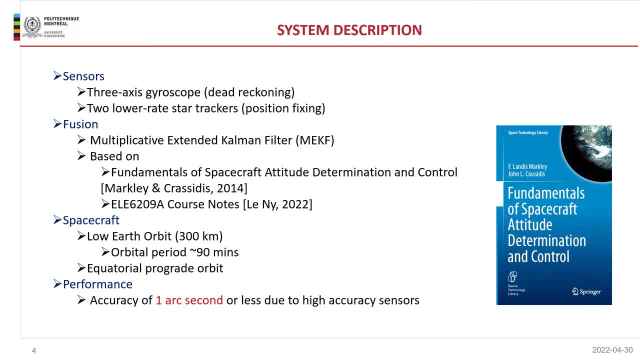 star trackers for position fixing. This combination of sensors is very popular in the space industry and it's very often seen on spacecrafts. We're going to fusion the measurements from the sensors using a multiplicative extended Kalman filter, The method that we used to develop this. 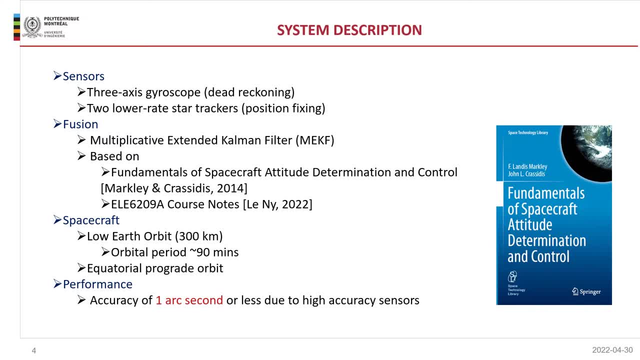 filter is based on the book on the right by Markle and Kresidis. It's a very thorough book. We also relied on the course notes. The satellite is in lower orbit, 300 kilometers of altitude. Its orbital period is 90 minutes. so that's going to be our simulation time. We're going to perform a simulation. 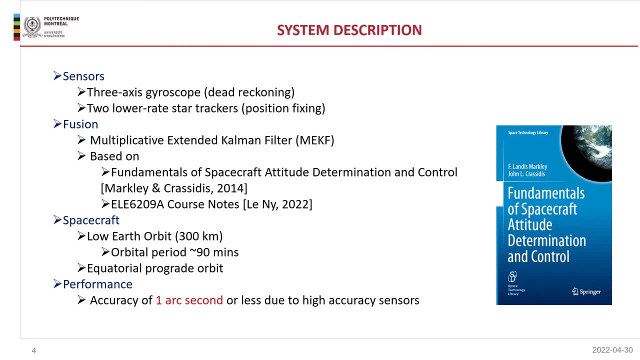 for one orbit. We've selected an equatorial prograde orbit. We're going to discuss in a minute what that means. More importantly, we expect the system to be accurate up to one arc second. That's mainly due to the high accuracy sensors that have been selected and that we're going to 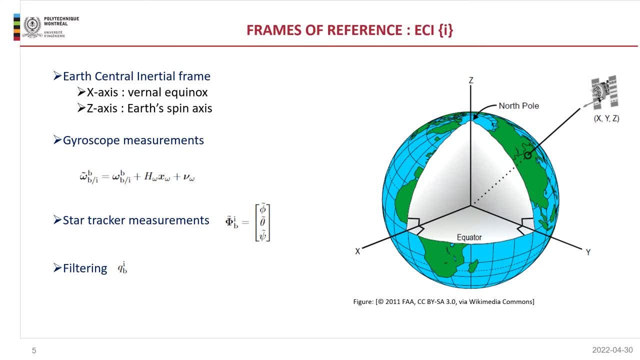 discuss in a minute as well. At this point in the term. we hope you're familiar with the ECI frame of reference. We still need to discuss it a little bit because it's really important in our process. For celestial applications. the star tracker measurements are reported with respect to the 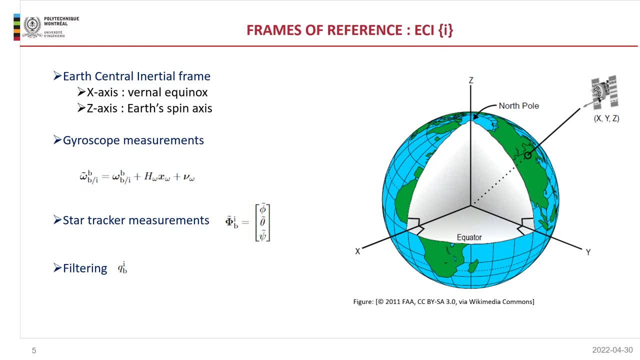 ECI frame and the gyroscope measurements are made with respect to the ECI frame as well. That's very convenient for us because we're going to do all our filtering and obtain the attitude quaternion in the ECI frame. The navigation frame is the orbital plane. 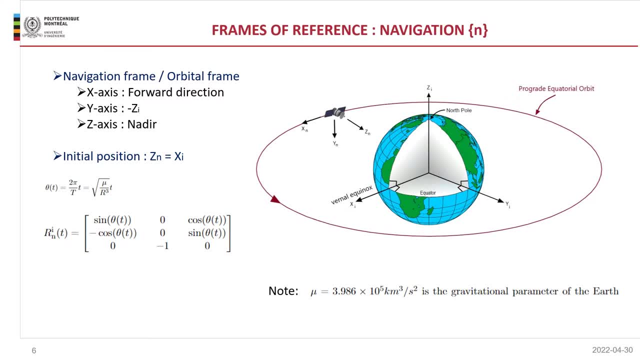 Since the topic of this project is really the navigation system, we didn't want to spend too much time on orbital mechanics, although we like that topic very much as well. To simplify our life a little bit, we selected an orbit that's going to help us. 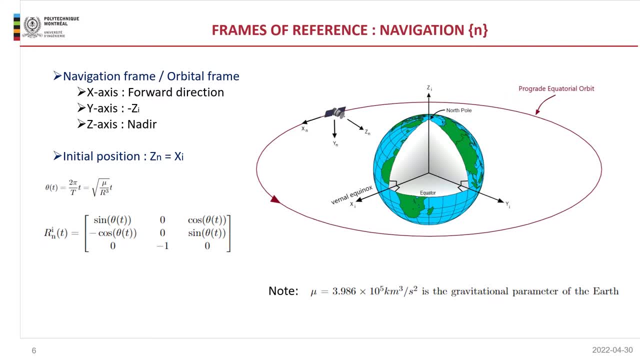 simplify the rotation matrix from I to N, We selected an equatorial prograde orbit. Prograde because this satellite turns in the same direction as the Earth. Since it's equatorial, the y-axis of the navigation frame is always parallel to the z-axis of the inertial frame. We end up with this nice rotation matrix on the lower left. 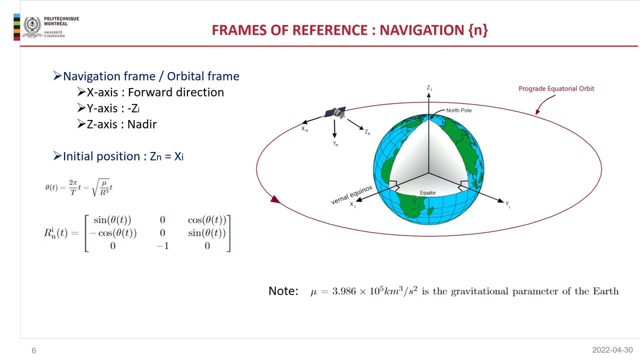 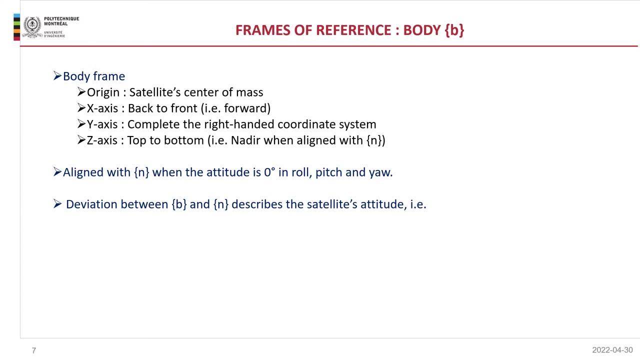 This is really a simplification, because as soon as the orbit is elliptical, then it's a little bit more cumbersome to come through the rotation matrix. The last frame of reference that we need to discuss is the body frame. The most important thing about the body frame is that it's perfectly aligned with the navigation frame when the 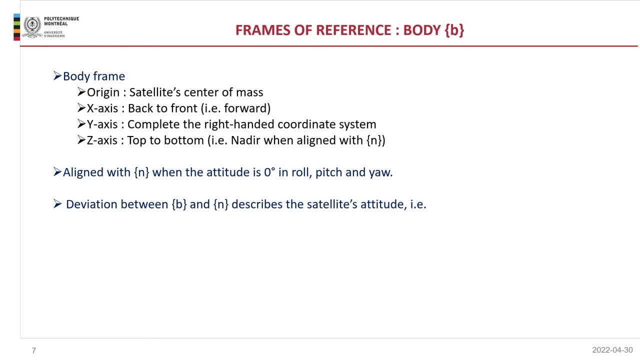 attitude is zero degree in roll pitch and er. For the rest, well, you know, the x-axis goes from the back to the front of the satellite and the z-axis points towards the Earth. But what does that mean, you know, for a satellite? What's the top of a satellite? 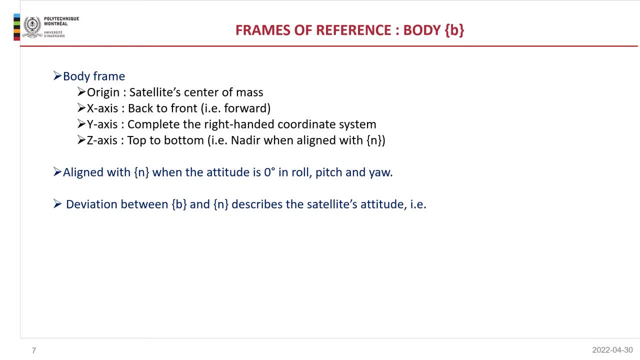 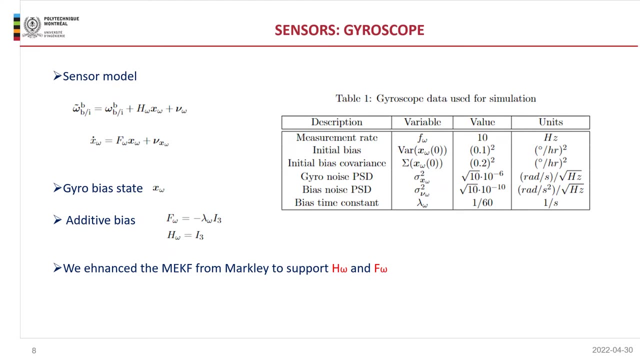 Well, luckily for us, we didn't need to model the dynamics of the system — of the satellite — we only needed the kinematics. So that doesn't really matter…. now Let's talk about the sensors. The first sensor is the gyroscope, and, fortunately for everybody, 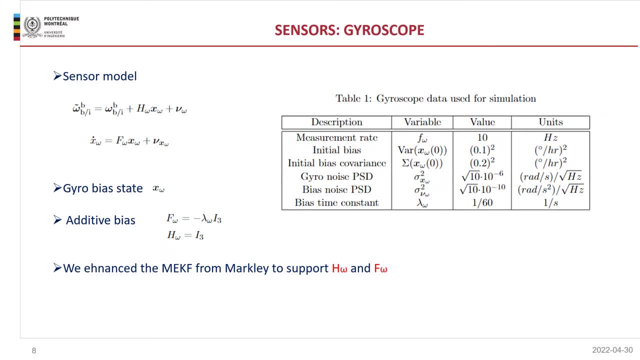 we modeled it the same way that we've seen in class, so you'll recognize the famous equation on the left. One important thing to mention is that the MEKF equations that were derived in the reference book for us did not include the lambda time constants for the bias, so we could 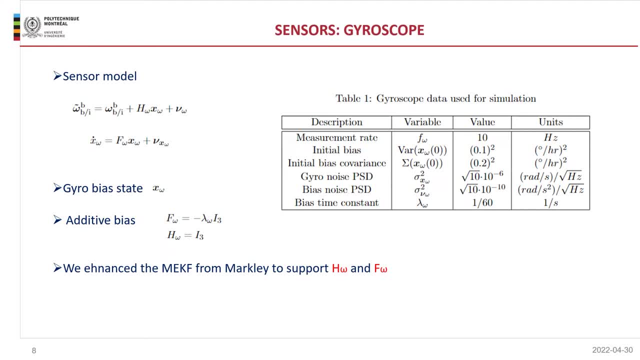 say that we enhanced the MEKF model from Markley and Cressidis, but they left us really good guidelines to do so. The data that was used for the simulation is shown in the table right there. It's a combination of data that was in the book and also that we found for specific. 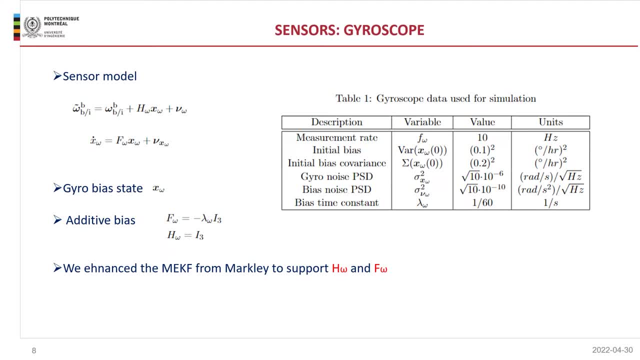 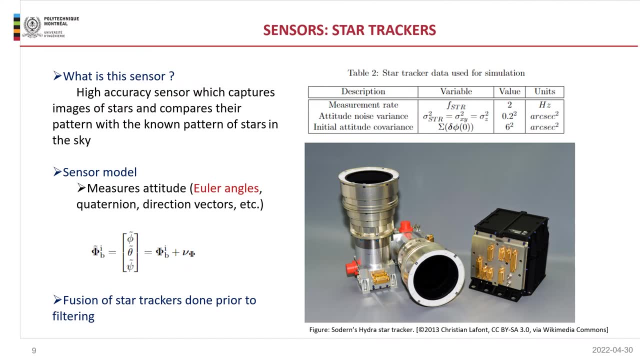 gyroscopes on spacecraft. The second type of sensors are star trackers. We've selected two star trackers for our system. We're going to discuss why on the next slide- but it's mainly for higher accuracy. Talking about accuracy, the star tracker is shown on the image as an accuracy of one arc second. It was developed by Southern Hydra. 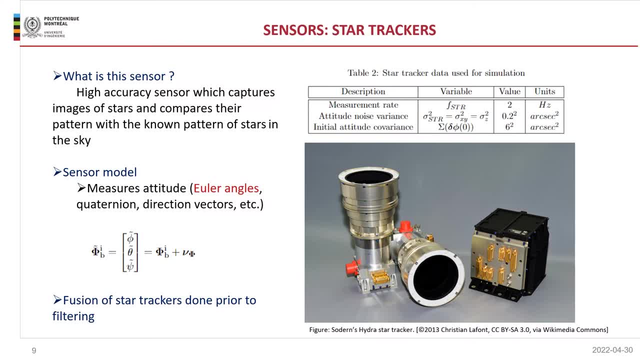 and it's already old. This photo was taken in 2013.. Modern star trackers or more modern star trackers or even more modern star trackers are more modern than modern star trackers. They have an accuracy of 0.2 or 0.1 arc seconds in all three axes. 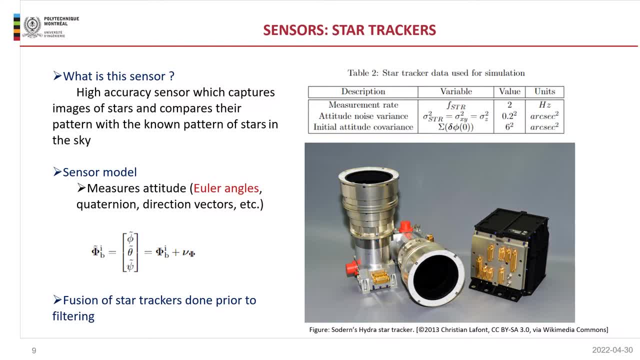 What is a star tracker? We've discussed it in class, but star trackers are high-accuracy sensors. They capture images of stars and they compare the pattern of the images with known pattern of stars that they have in their catalog. They determine the attitude of the body frame with respect to the 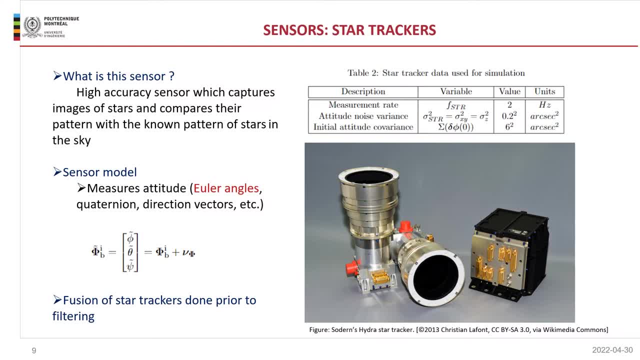 ECI frame. based on that, They report measures in the form of Euler angles, quaternions or direction vectors. For our project, we've decided to work with Euler angles. Now we have two star trackers, but we've decided to fusion them before doing the filtering. 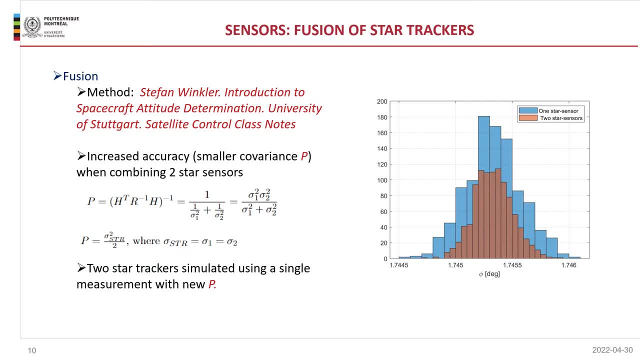 and that's what we're going to discuss now. There are multiple ways to fusion star trackers for Kalman filtering. but Haram has had a class in Germany by Dr Stephen Winkler. It's a class about spacecraft attitude determination and in class they specifically discuss the topic. 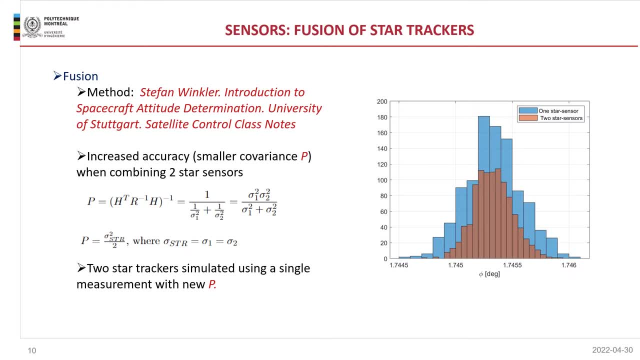 There's a simple math involved in combining measurements from two different star trackers with the same covariance and you basically end up with covariance divided by two, so you have better accuracy. To prove that, we've performed some Monte Carlo simulations and, as you 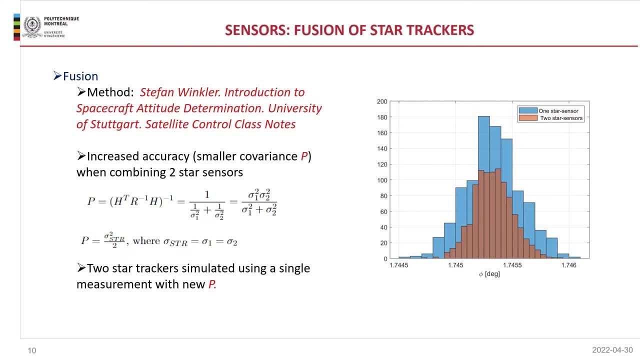 can see on the image, when you have one star tracker your covariance is higher, but when you have two star trackers it's much more accurate. So we've done some Monte Carlo simulations and, as you can see on the image, when you have one star tracker your covariance is higher, but when you have two star trackers it's much more accurate. 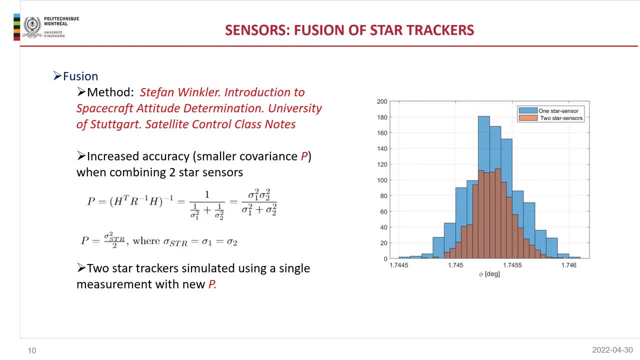 It's reduced, so you have higher accuracy, and that's the method that we were going to employ before Kalman filtering. We're basically saying that we have two star trackers and we can assume that we have a single measurement update with the covariance. 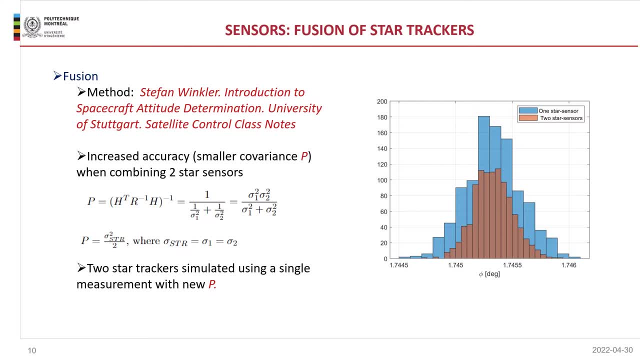 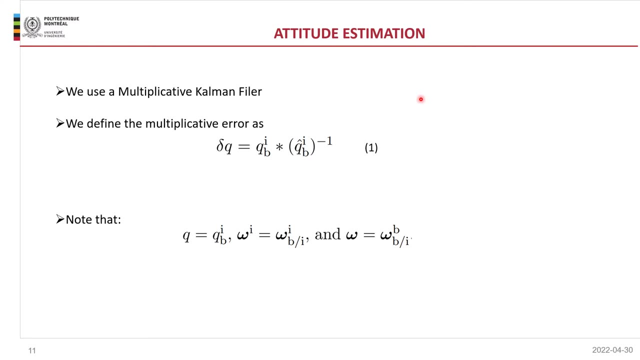 of the single star tracker, divided by two. Now it's time to discuss the Kalman filtering, and my colleague Haram is going to take over. Now we want to describe our proposed solution to fuse the data of the gyro and the two star trackers. 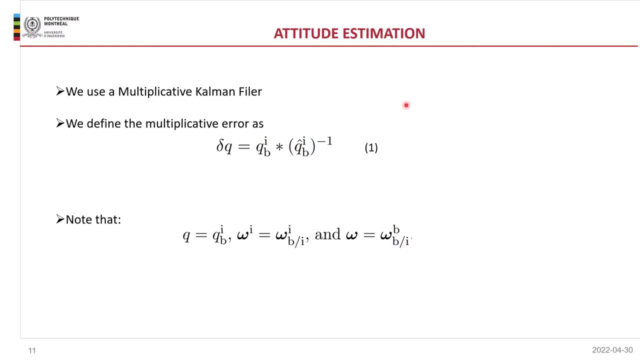 The goal is to estimate the attitude. Our approach is based on the multiplicative extended Kalman filter. So the goal of the filter is to estimate the quadrillion which describes the rotation from frame E to frame B. In order to do that, we define a multiplicative error, as expressed in equation 1.. 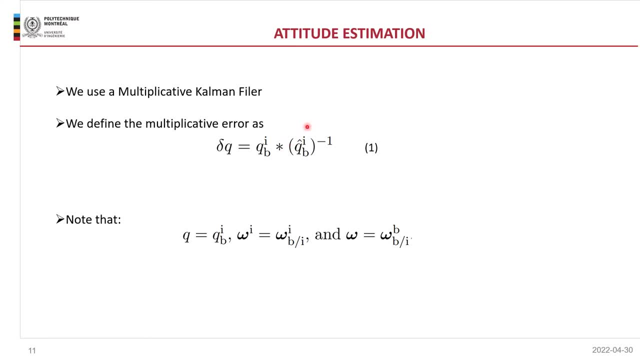 Before starting with equations of the Kalman filter. we note that we use those notations to simplify our equations. We note that we use those notations to simplify our equations. So now we want to describe our proposed solution to fuse the data of the gyro and the two star. 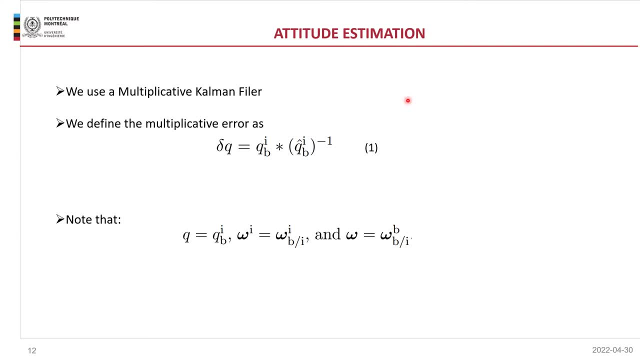 trackers. The goal is to estimate the attitude. Our approach is based on the multiplicative extended Kalman filter. So the goal of the filter is to estimate the quadrillion which describes the, which describes the rotation from frame E to frame B. 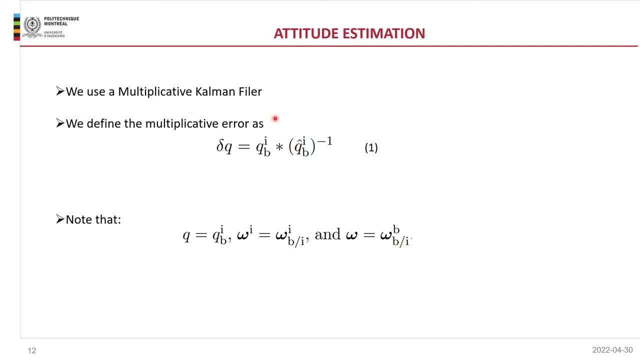 In order to do that, we define a multiplicative error, as expressed in equation 1.. Before starting with the equations of the Kalman filter, we note that we use this notation to simplify our equations In order to obtain the mechanization equations. 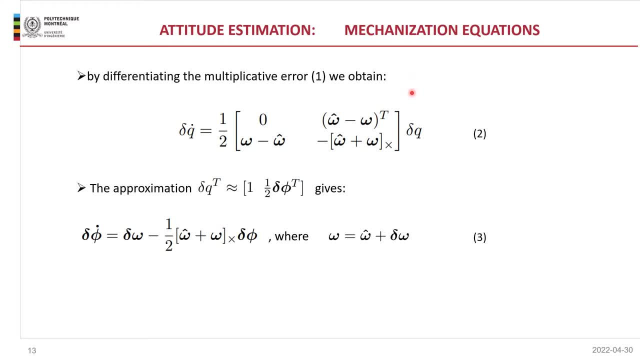 we differentiate the multiplicative error described above. So we find equation 2, where omega is the true angular rate and omega hat is the estimated angular rate. Then we make this approximation so that the three last components of the quaternion error are the angular error. now 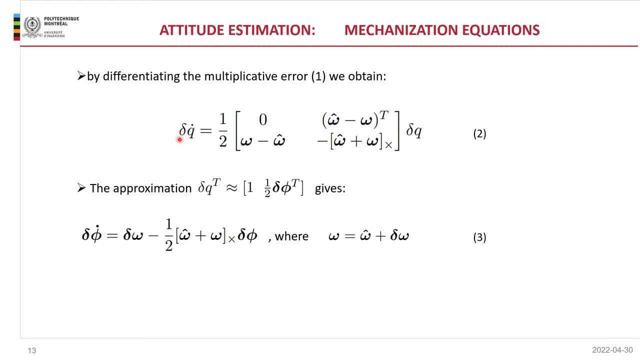 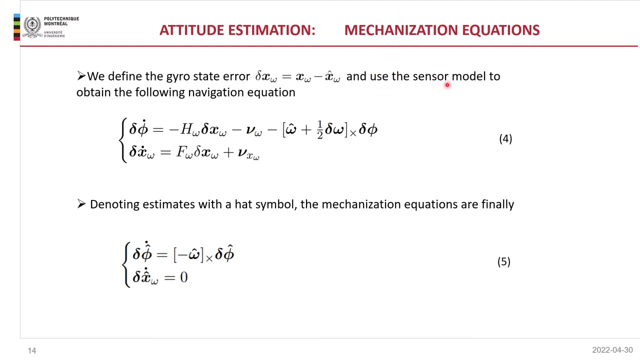 And then from the three last lines from equation 2, we find the equation 3, where delta omega is the angular rate error, By using the sensor model described above and by defining the gyro state error, delta x, omega- as the error between the true gyro state. 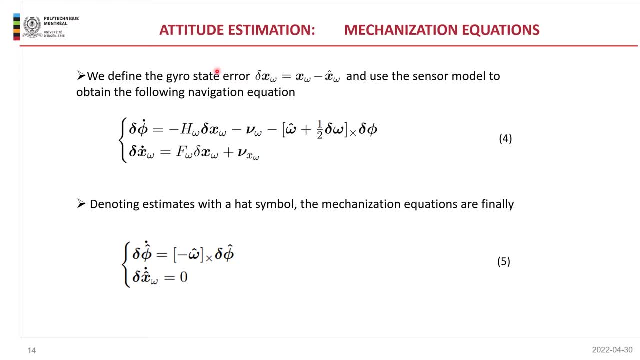 and the true gyro state, we obtain the following navigation equation, described in 4.. Now we are denoting the estimates with the hat symbol and we set the error vectors to 0. So we obtain the equation 5, which are the mechanization equations needed for the Kalman filter. 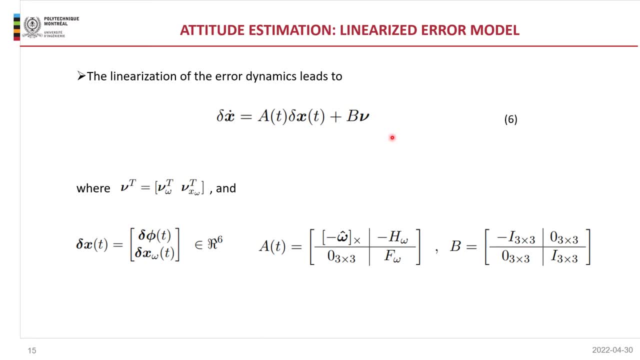 Before describing our algorithm, we have to linearize our system, Our error model. So, after linearizing the dynamics, we obtain the following equation 6, so that our state vector is an error state vector which is composed by the minimized quaternion error, delta phi. 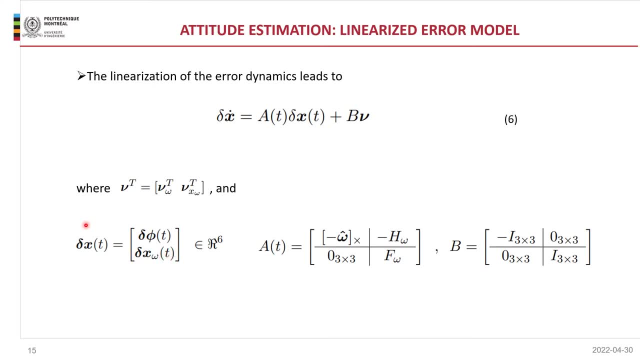 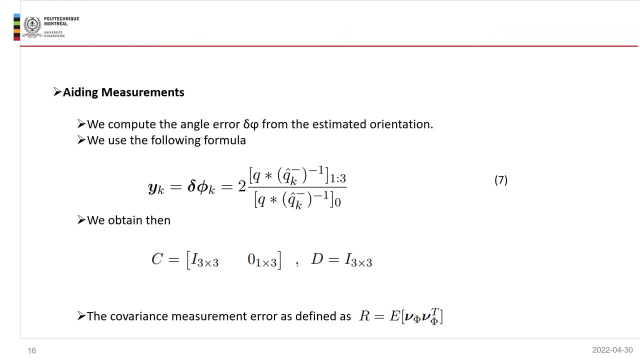 and the gyro state error delta x. So the state error contains six components. The measures from the star trackers are Euler angles. To update our estimate, we transform the Euler angles to attitude quaternion Q And then we compute the angle error delta phi. 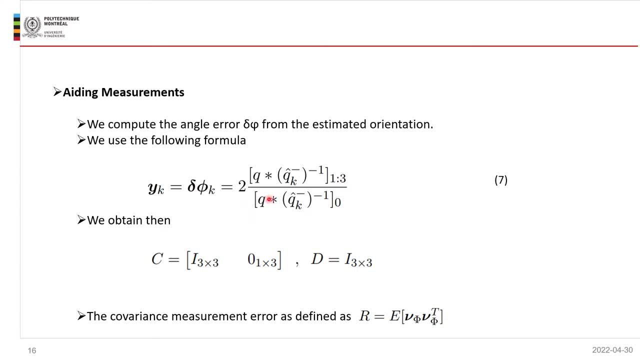 by using this equation. So, as we can see, this equation is linear in delta x. We obtain then C and D as follows. The measurement covariance matrix R is a 3x3 matrix of the attitude measurement error angles. We assume that R is the covariance matrix. 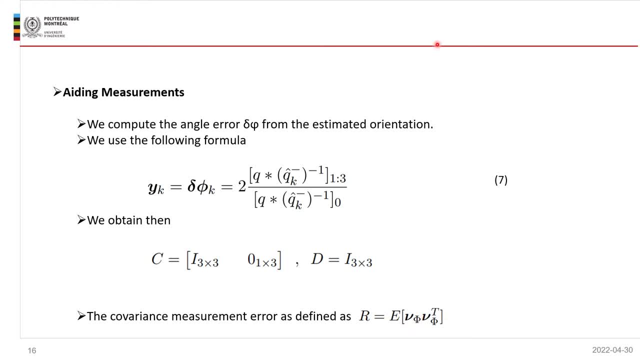 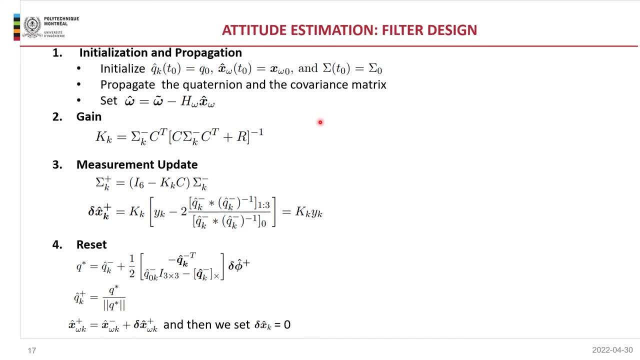 from the noise vector of the star trackers. So now, after linearizing our system, we can describe our filter design. Our filter design can be summarized in four steps. The first step: we have to initialize first the quaternion, the bias and the covariance. 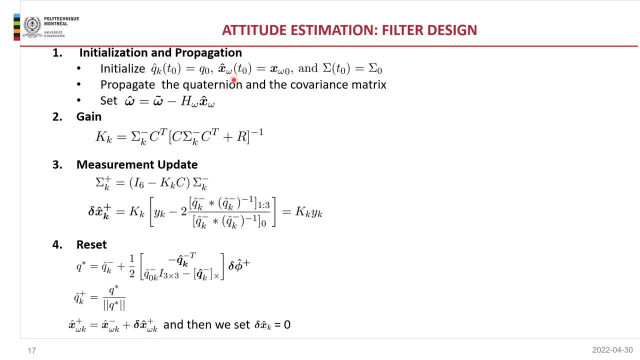 And by using this initialization we can propagate our quaternion and covariance matrix. So first, for example, for the quaternion, we integrate, we integrate the quaternion kinematics equations by using the initial value, And then we set the omega hat, which is the estimated angular rate. 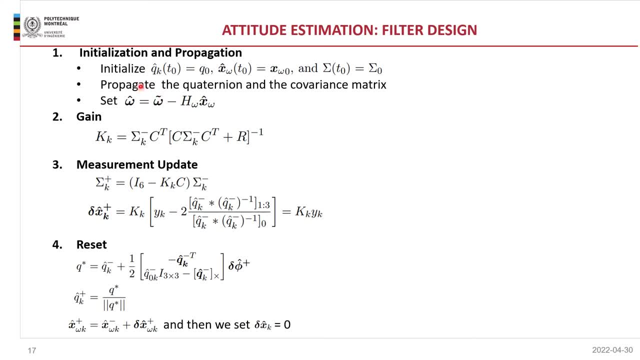 as follows: After the first step, after initialization and propagation, we can now calculate or compute our gain K, which is the Kalman gain, And once we have our gain, we can update. we can update the covariance matrix and the error state vectors as follows: 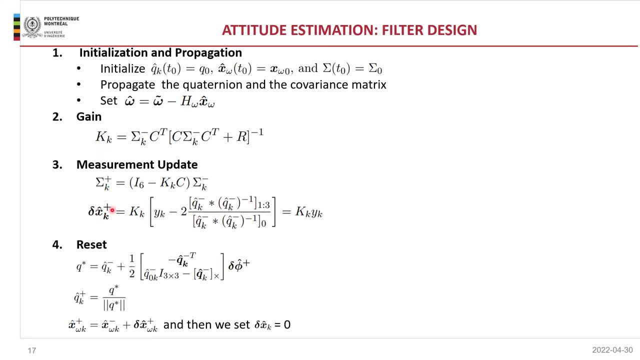 And, as we see, as we see here, our multiplicative extended Kalman filter estimates the error state and not the quaternion. Once we have an estimate for the error, we can- we can update the attitude quaternion and the gyro state. So we can now. 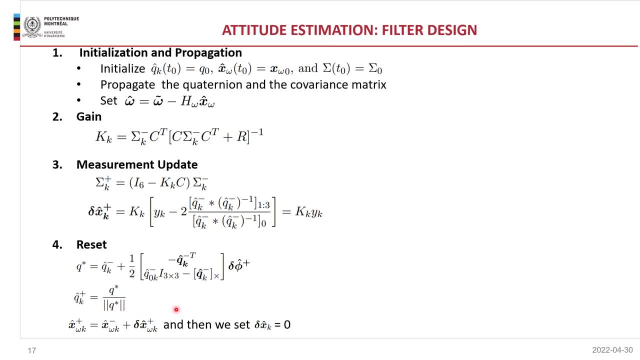 we can now reset, And after that we have to reset our delta x, We have to reset our error state vector to zero And then, after resetting the value to zero, we can repeat all the steps, starting from one to four And taking those estimates as initial values. 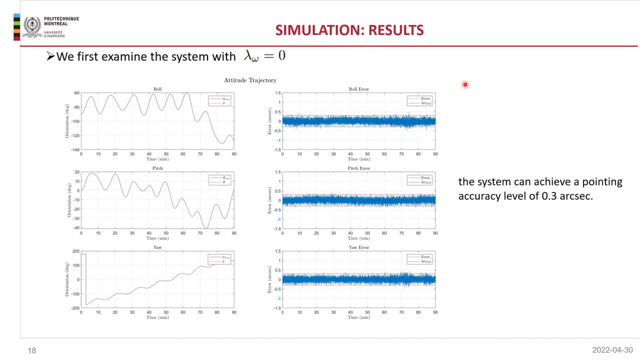 We present and analyze now our results. The diffusion of the star trackers and the gyro using the multiplicative extended Kalman version described above, provides an estimate of the satelizer attitude and the gyroscope biases. So first we examine the system's behaviors. 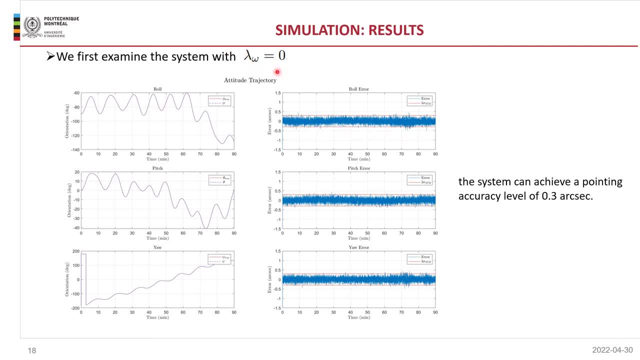 with lambda. lambda equals zero For the attitude estimation. we see in this figure that the filtered data follows the true error angle. The attitude error plots indeed show that the state that the system can achieve a pointing accuracy level of the zero three. 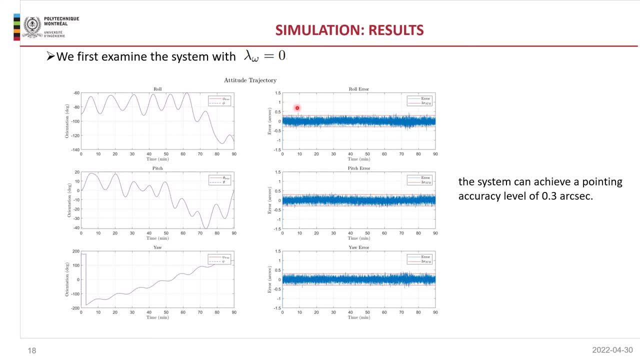 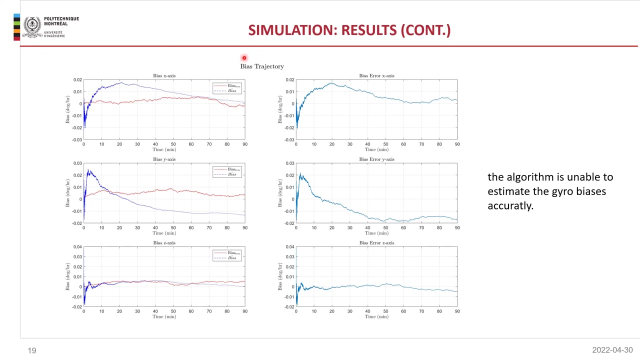 of about zero, three arc second. So the red curves in the error plots corresponds to the three sigma of the star tracker. We have to note that those lines have been plotted for reference only and don't provide information on the statistics of the error. Here we represent our 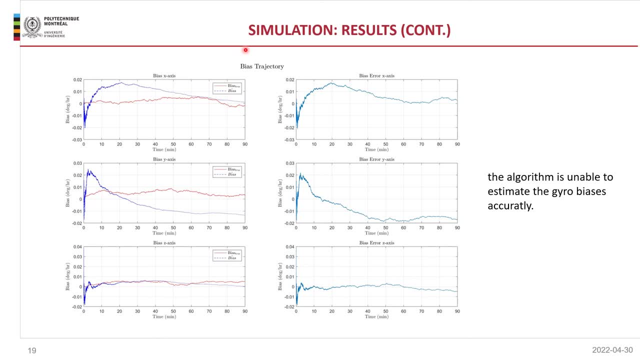 in those plots we represent our bias estimations. So the red one is the true bias and the blue one is the estimated bias And, as we see, the algorithm is enabled to approximate the bias. Here, for example, is the bias error. 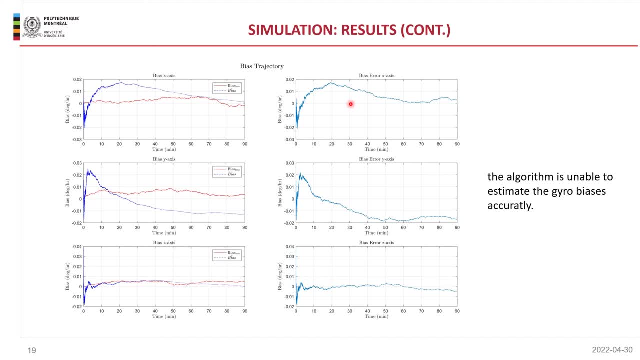 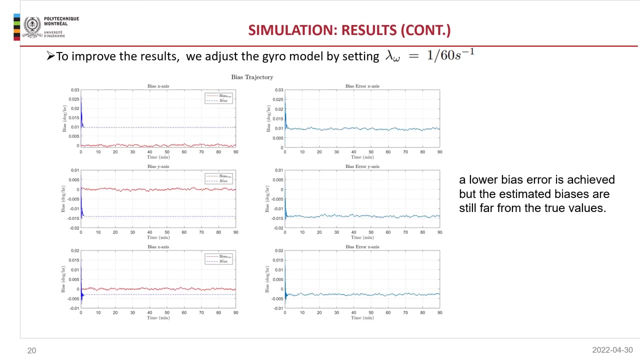 And, as we see, the bias doesn't converge and ROCH from the expected bias zero And due to this problem, we are actually enabled to determine the attitude accurately for simulations longer than two hours, As the system after two hours becomes unstable. In order to improve our results, 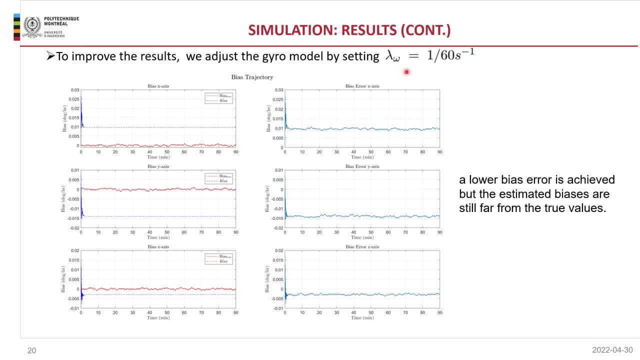 we thought about adjusting the gyro model by setting lambda different from zero, And those are our results for the bias And, as we see here, those figures demonstrate that the lower bias error is achieved, but the estimated biases are still far from the true values. 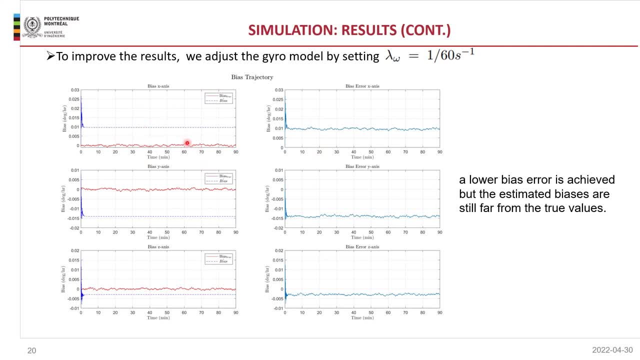 So the blue one are the estimated bias and the red one are the true bias. The accuracy of the attitude estimation is also slightly improved. So we didn't mention here because it's slightly improved but it's still unstable for longer simulation periods. So in summary, 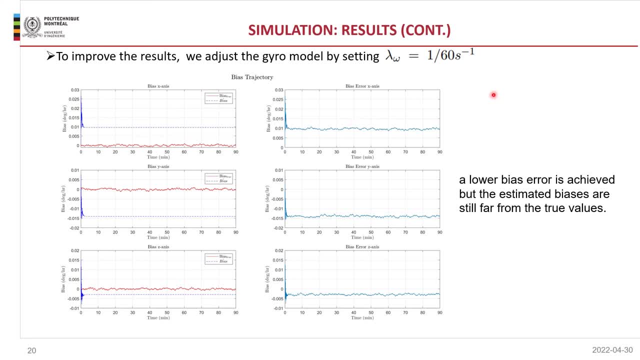 we can affirm that the navigation system generates acceptable attitude estimates for the period of interest which corresponds to an orbit. However, we recommend to improve or adjust the gyro model. The results show that a good bias estimate is crucial for performance. extended Kaman filter. 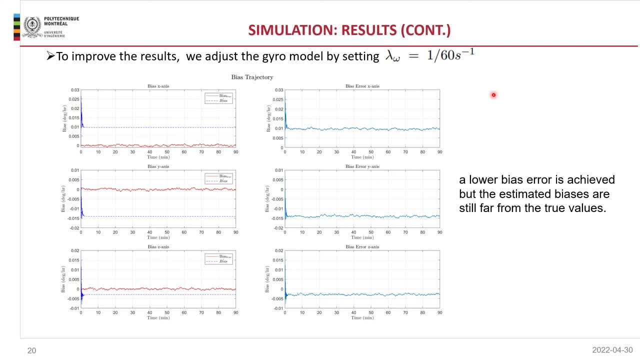 And in our case we need to calibrate the system after each orbit to ensure acceptable filter outputs, Because for simulation longer than 90 minutes is difficult to achieve acceptable performance without adjusting the gyro parameters. We've already reached the end of the presentation. 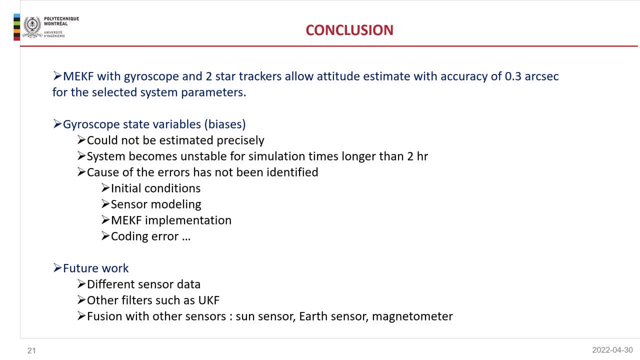 We've shown that MEKF with one gyroscope and two star trackers allows an attitude estimation with an accuracy of 0.3 arc seconds. But we've also shown that we encountered some problems during our simulation. Mainly, we were not able to estimate correctly. 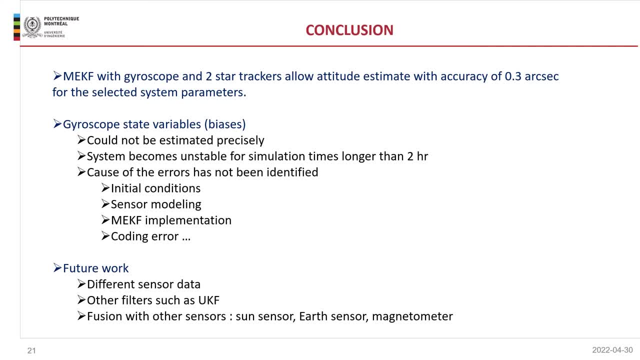 the biases of the gyroscope. So what was the problem? Well, we're not sure. It could be initial conditions, the modeling of the sensor, the implementation of the MEKF. and we're not ruling out coding errors, although we haven't found any, of course.